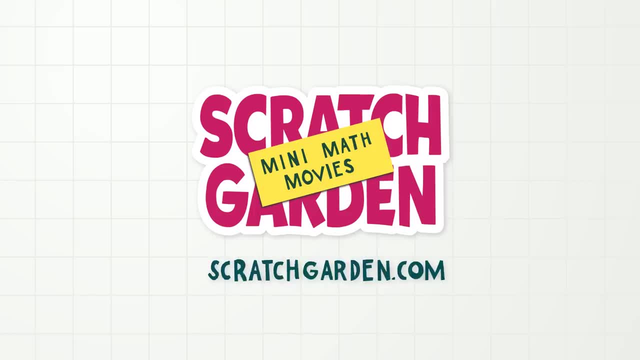 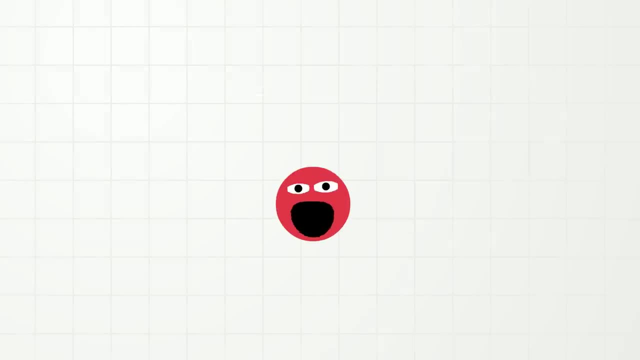 Oh, hi everybody. Today I am going to talk to you about numbers And measuring And maybe even salamanders. I really like salamanders. So one thing we use numbers for is when we are measuring. Measuring is finding out the size of something or the amount of something. 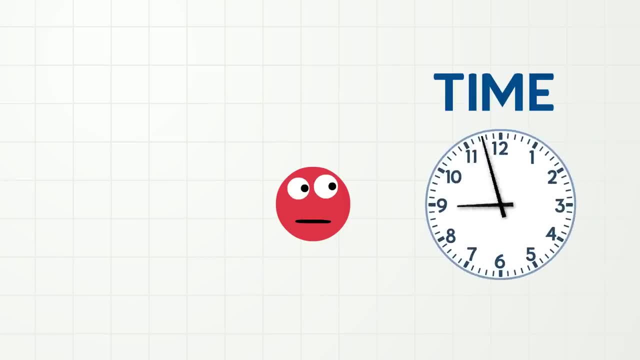 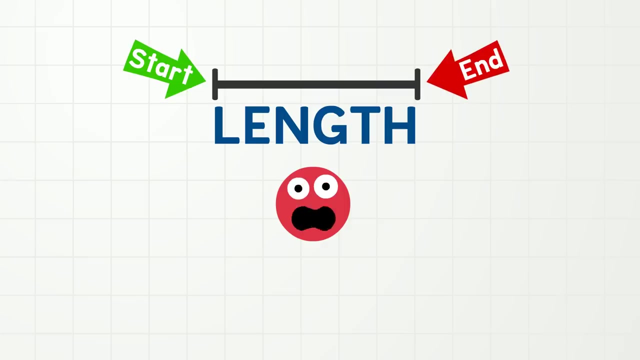 And we can measure many things like time, weight, temperature or even speed, But today we are going to measure length. Length is the distance between two points, like how far it is between the start and the end of something, And we measure length to find out. 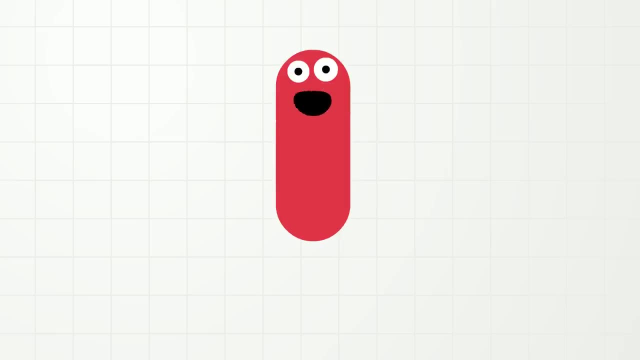 how long something is, And also how tall or wide or even how far away something is. Ok, this might be a little confusing, so why don't we take a break and have a snack? Hum, hum, Ok, that's enough. Anyway, when we measure the length of something, we measure. 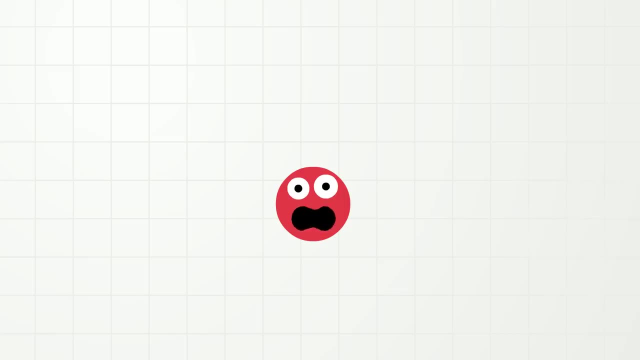 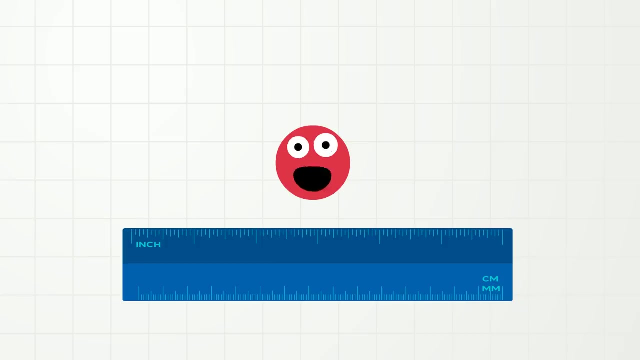 with units, Units. There are many standard units that you can use like inches or centimeters. There are also many non-standard units that you can use like paper clips. Today, I want to use my favorite non-standard unit: the salamander. It's a salamander. 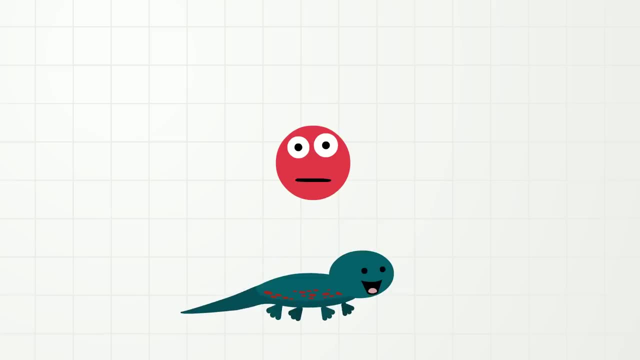 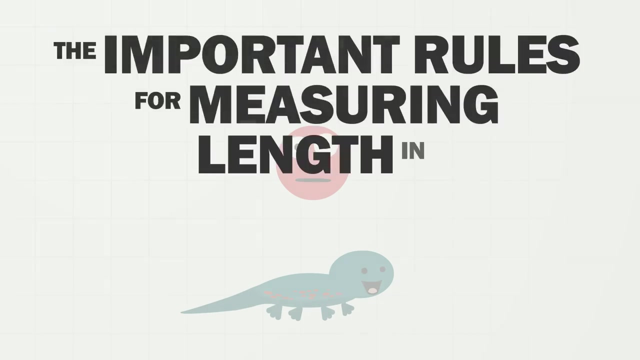 So right now, salamander is going to be a unit that we can count and use to measure things, But before we do that, we need to talk about the rules for measuring, which leads us to a new segment called The Important Rules for Measuring Length in Straight Lines with Non-Standard Units. 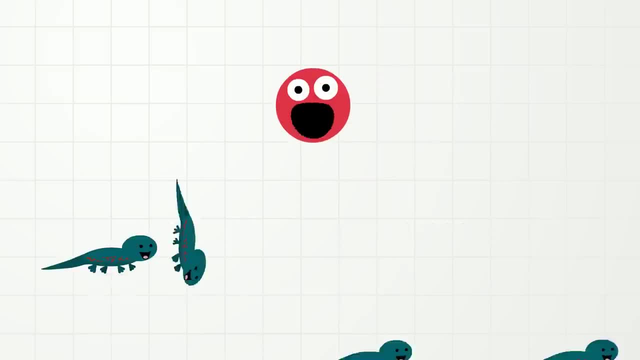 Wow, that is a long title. Rule number one: All of the units need to be the same size and direction. Sorry, super tiny salamander, Sorry, turtle. Rule number two: All of the units should touch each other at the ends, but not overlap on top of each other. 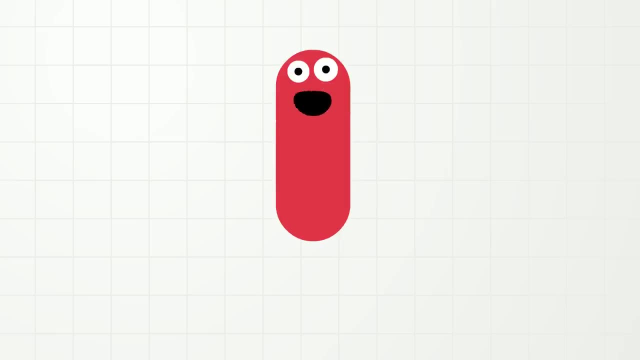 how long something is, And also how tall or wide or even how far away something is. Ok, this might be a little confusing, so why don't we take a break and have a snack? Hum, hum, Ok, that's enough. Anyway, when we measure the length of something, we measure. 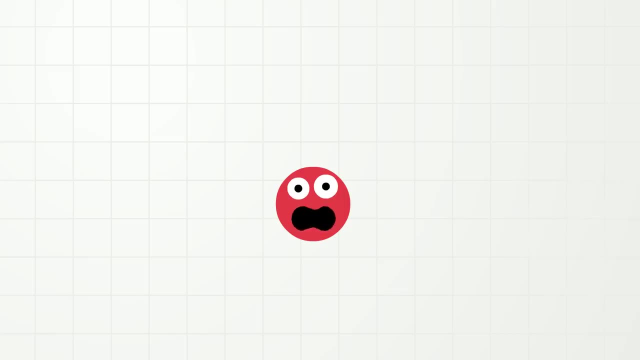 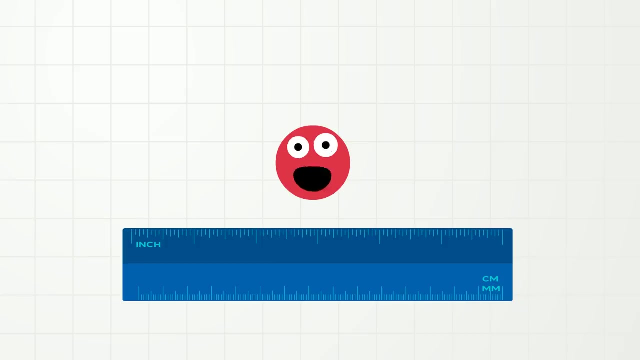 with units, Units. There are many standard units that you can use like inches or centimeters. There are also many non-standard units that you can use like paper clips. Today, I want to use my favorite non-standard unit: the salamander. It's a salamander. 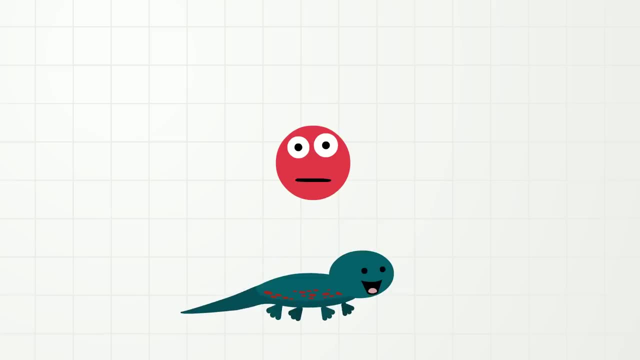 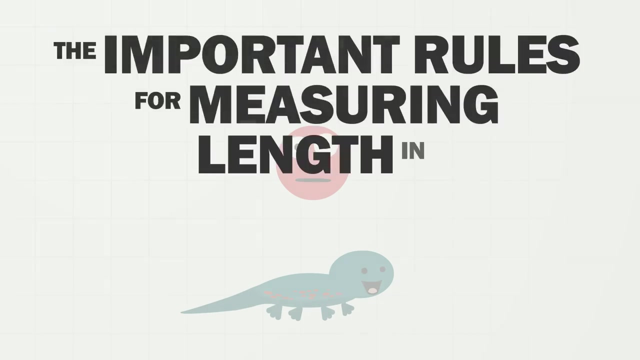 So right now, salamander is going to be a unit that we can count and use to measure things, But before we do that, we need to talk about the rules for measuring, which leads us to a new segment called The Important Rules for Measuring Length in Straight Lines with Non-Standard Units. 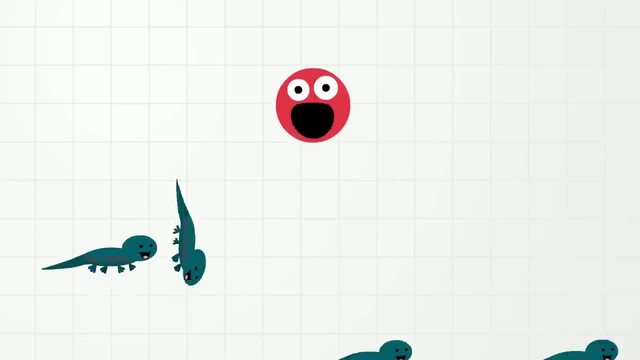 Wow, that is a long title. Rule number one: All of the units need to be the same size and direction. Sorry, super tiny salamander, Sorry, turtle. Rule number two: All of the units should touch each other at the ends, but not overlap on top of each other. 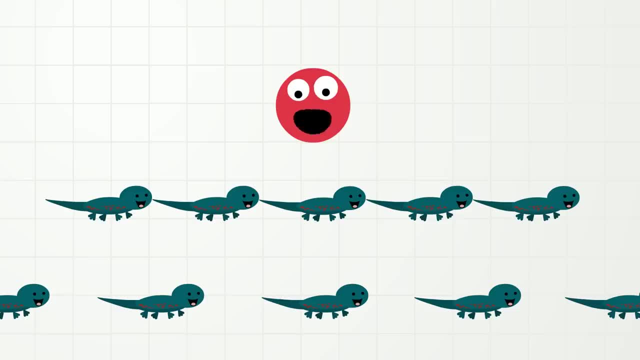 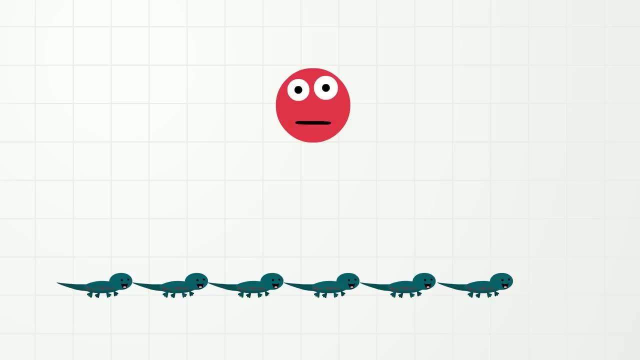 And they should also not be spread out. Salamanders, come back. Rule number three: Usually the units need to make a straight line like this, but not like this. And rule number four: When measuring something, for example the length of this book, we start. 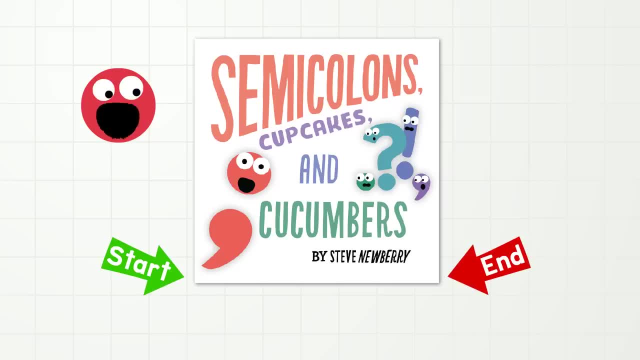 the units next to one end of the book and finish at the other end of the book, like this. So we don't start from the center of the book and we don't start from over here or in some other place, like the beach. 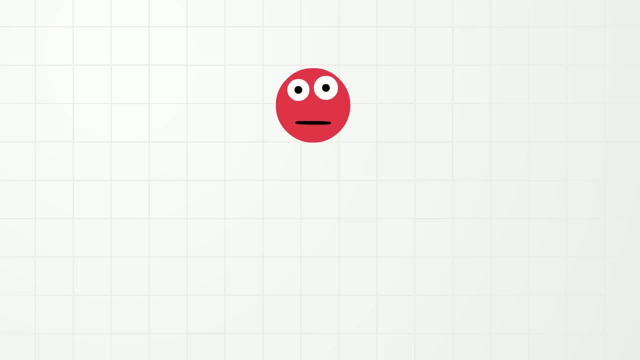 Okay, that now ends the part of the show called The Important Rules for Measuring Length in Straight Lines with Non-Standard Units. Okay, so now let's do some measuring. First, we need something to measure. What should we use? 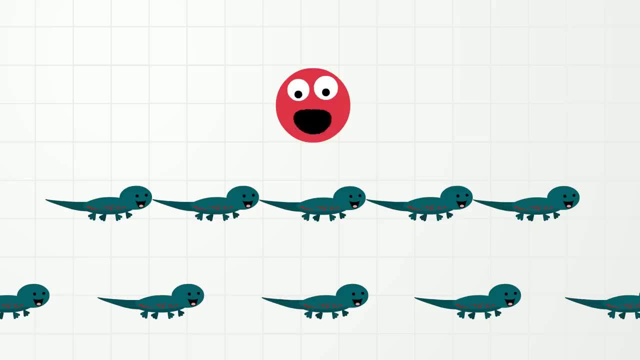 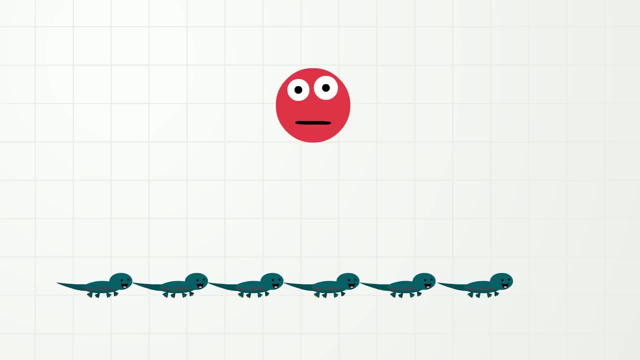 And they should also not be spread out. Salamanders, come back. Rule number three: Usually the units need to make a straight line like this, But not like this. And rule number four: When measuring something, for example the length of this book, we start. 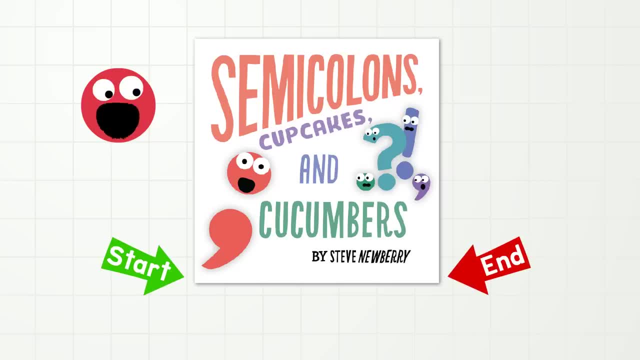 the units next to the lines, next to one end of the book and finish at the other end of the book, like this. So we don't start from the center of the book and we don't start from over here or in some. 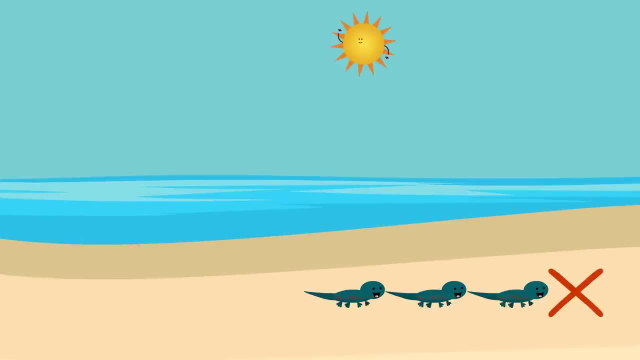 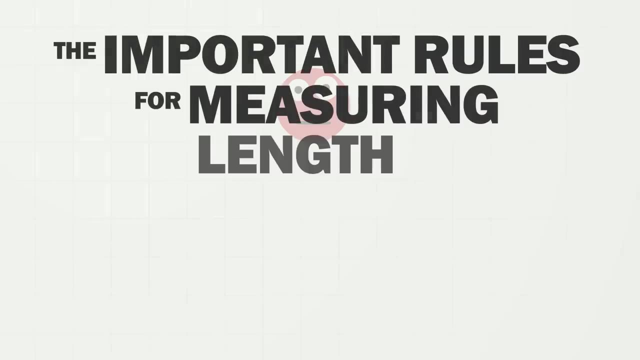 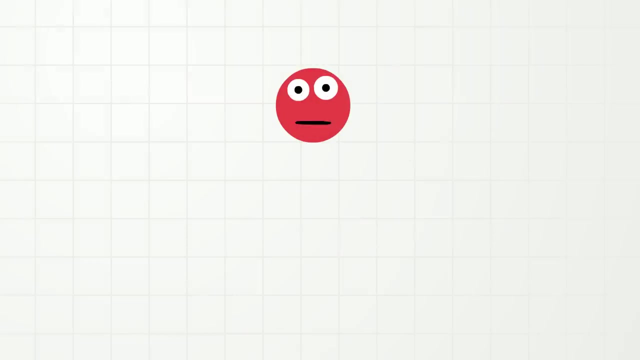 other place, like the beach. Okay, that now ends the part of the show called The Important Rules for Measuring Length in Straight Lines with Non-Standard Units. Okay, so now let's do some measuring. First, we need something to measure. 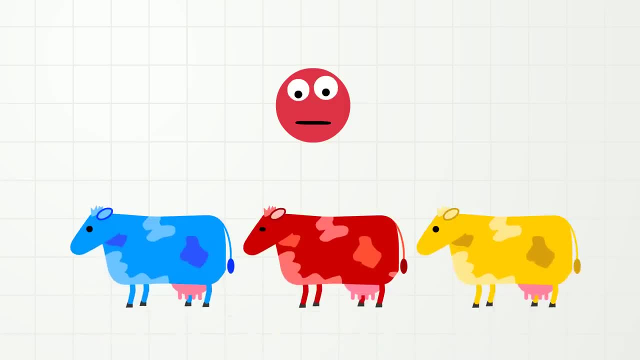 What should we use? Oh, I know how. about cows With funny hats? ha, Okay, here we have three cows- Blue cow, red cow and yellow cow- And they all have funny hats. But I want to know which cow has the tallest hat. 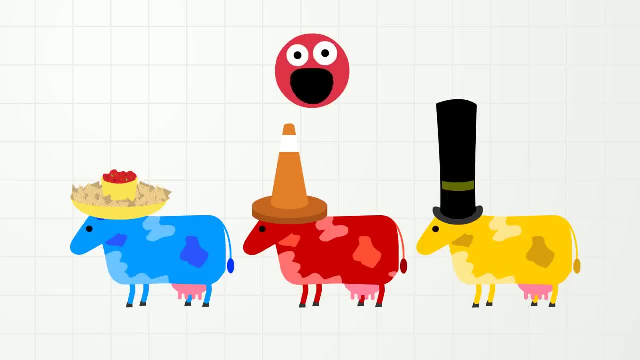 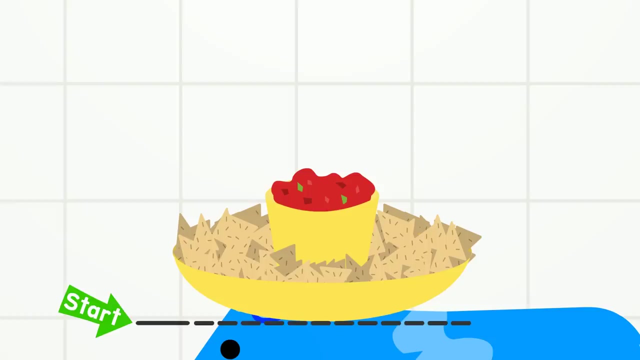 So we will have to measure. We will measure the length, or some might call it the height of each cow's hat, And first up is blue cow. Let's measure the height of blue cow's hat with salamanders. Remember, we start measuring at one end of the hat and go in a straight line next to. 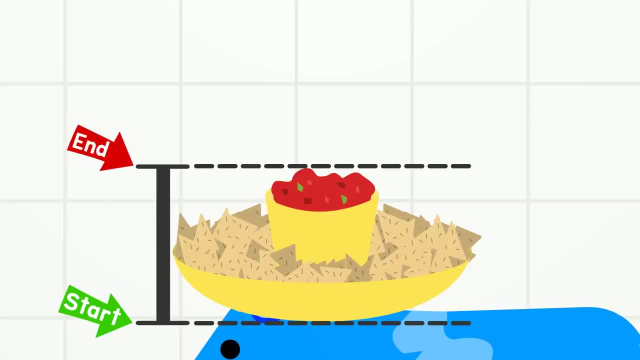 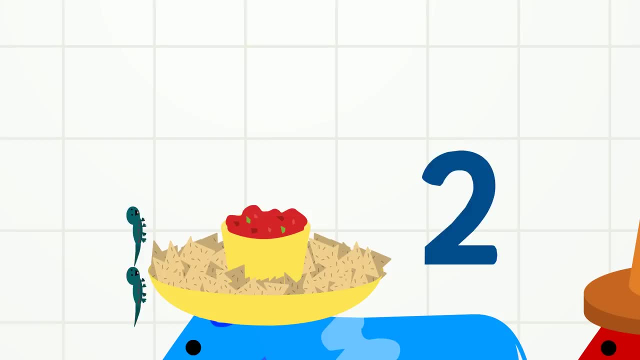 the hat all the way to the other end of the hat. So blue cow's hat is one, two salamanders long, And blue cow's hat is three, Two salamanders long, Or we can also say two salamanders high. 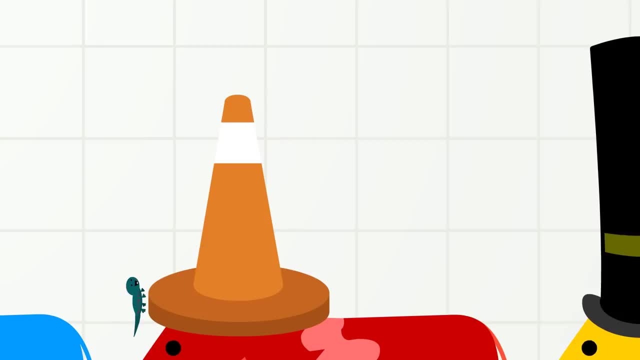 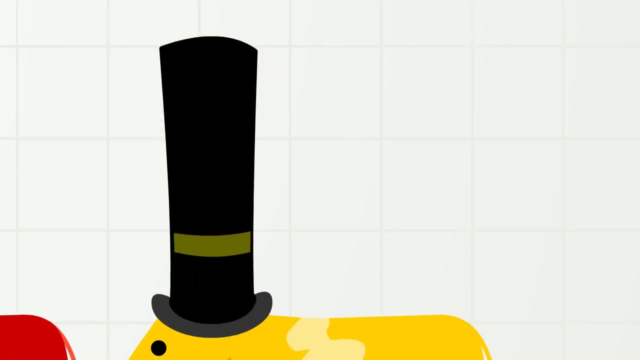 Okay, red cow. Red cow's hat is one, two, three, four salamanders long, Or we can also say four salamanders high. And last is yellow cow. Yellow cow's hat is one, two, three, four, five salamanders long. 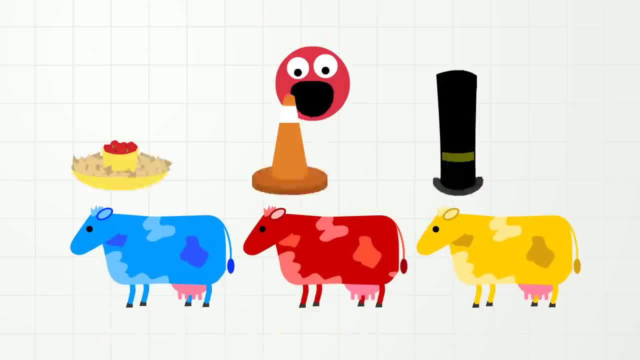 Oh, I know how about cows With funny hats? ha Okay, here we have three cows: Blue cow, red cow and yellow cow, And they all have funny hats. But I want to know which cow has the tallest hat. So we will have to measure. 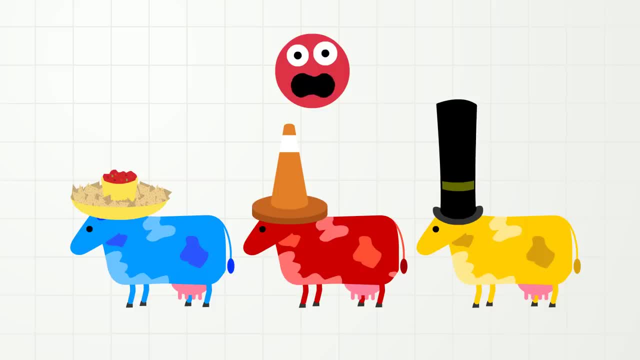 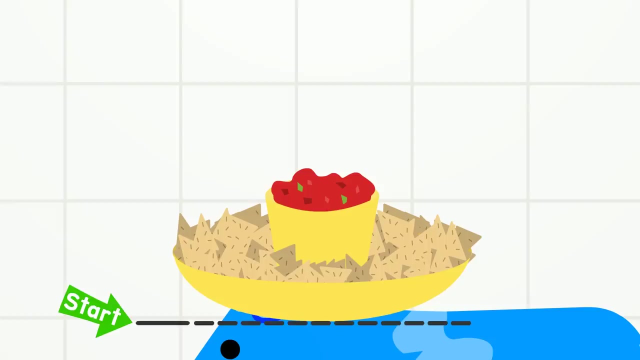 Let's measure the length, or some might call it the height of each cow's hat, And first up is blue cow. Let's measure the height of blue cow's hat with salamanders. Remember we start measuring at one end of the hat and go in a straight line next to. 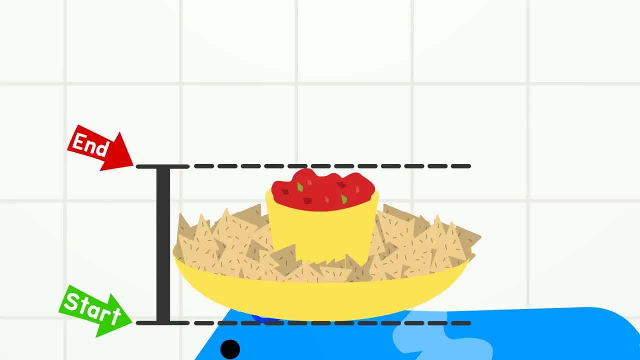 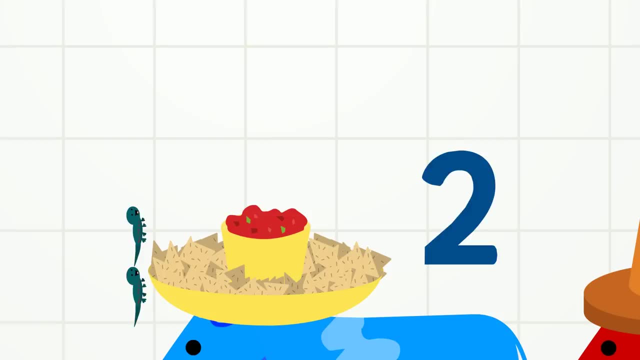 the hat all the way to the other end of the hat. So blue cow's hat is one, two salamanders long, And blue cow's hat is three, And blue cow's hat is four And blue cow's hat is five. 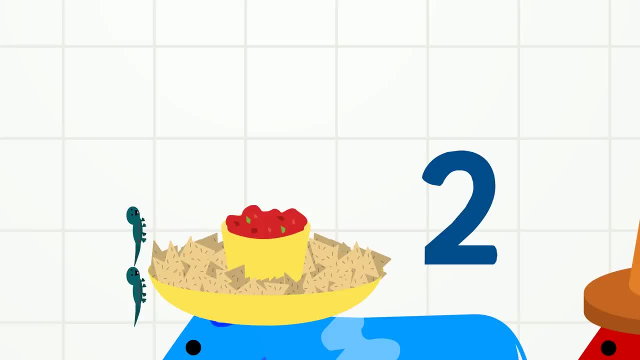 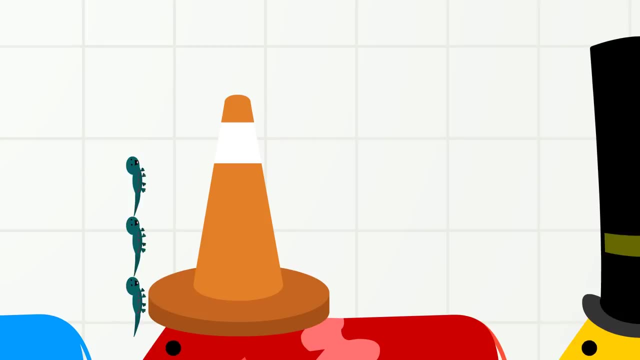 Or five salamanders long, Or we can also say two salamanders high. Okay, red cow, Red cow's hat is one, two, three, four salamanders long, Or we can also say four salamanders high. 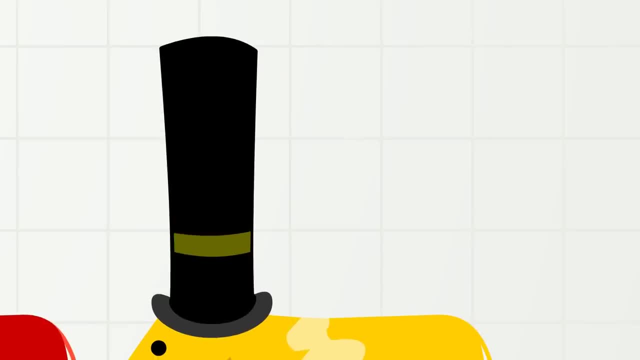 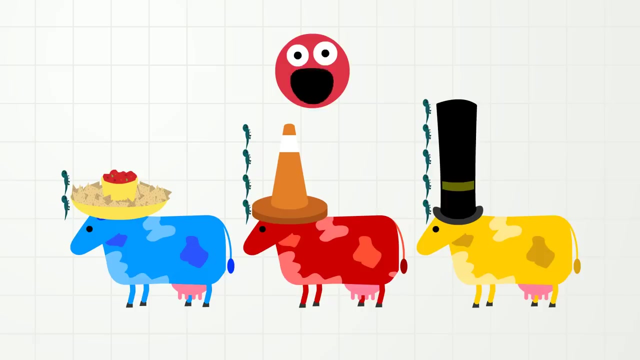 And last is yellow cow. Yellow cow's hat is one, two, three, four, five salamanders long. Yellow cow's hat is five, four, We can also say five salamanders high. Now let's compare hats. but first snack time. 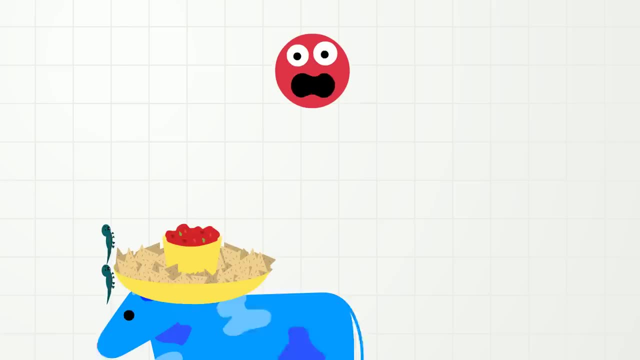 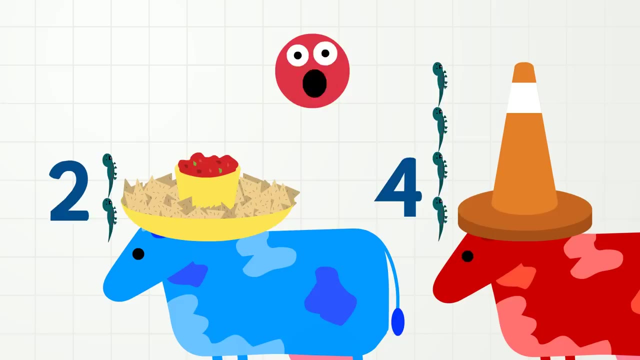 Hum, Hum. Okay, that's enough. So blue cow's hat is two salamanders high and red cow's hat is four salamanders high. Four is a larger number than two, so that means that red cow's hat is taller than. 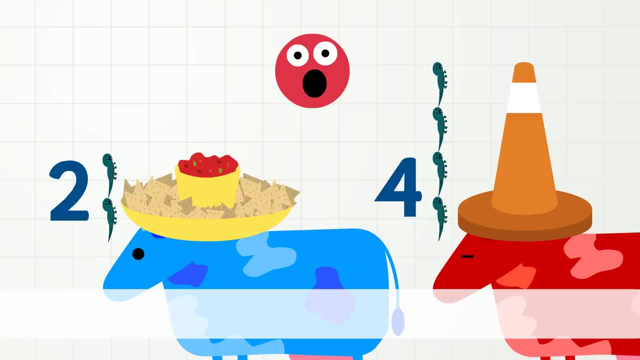 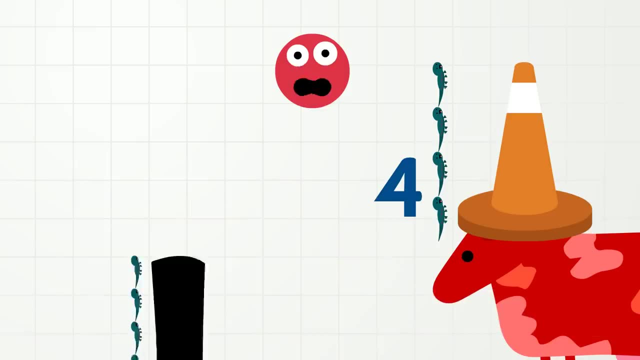 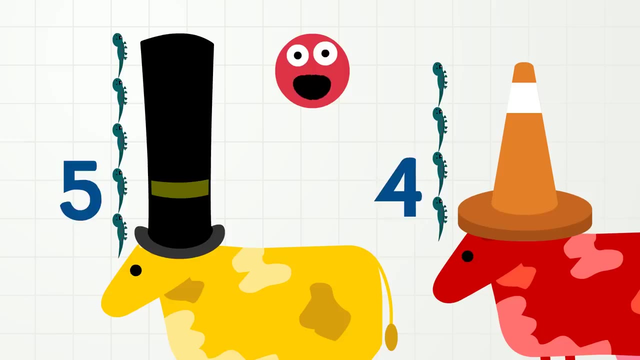 blue cow's hat, And the opposite is also true. Blue cow's hat is shorter than red cow's hat. Now if we look at yellow cow's hat, it is five salamanders high Five is a larger number than four, so this means that yellow cow's hat is taller than. 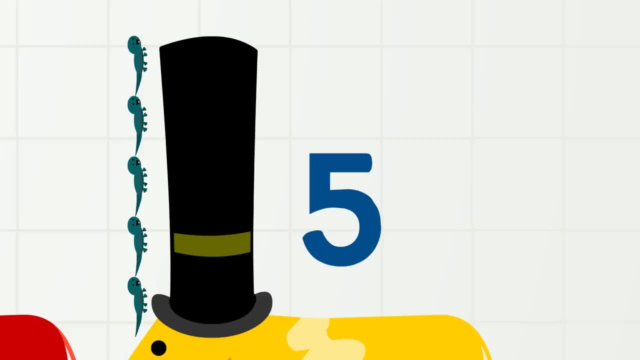 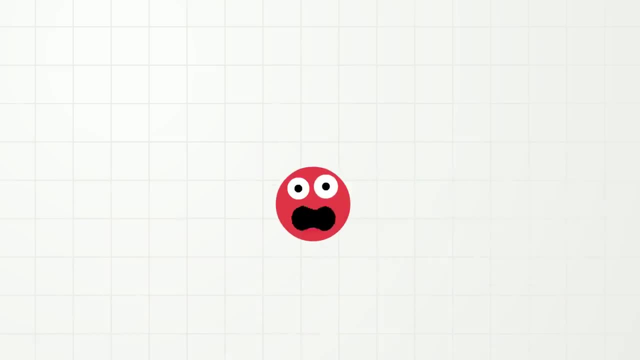 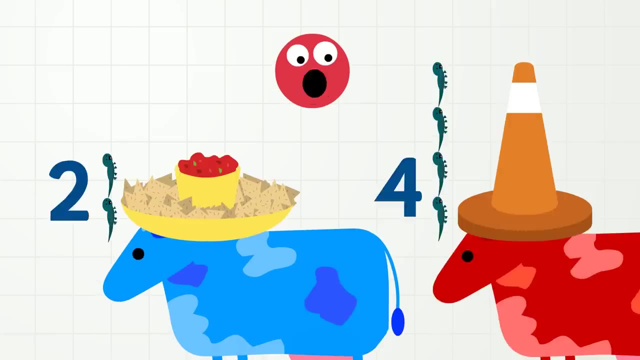 Or we can also say five salamanders high. Now let's compare hats, But first snack time. Okay, that's enough. So blue cow's hat is two salamanders high And red cow's hat is four salamanders high. 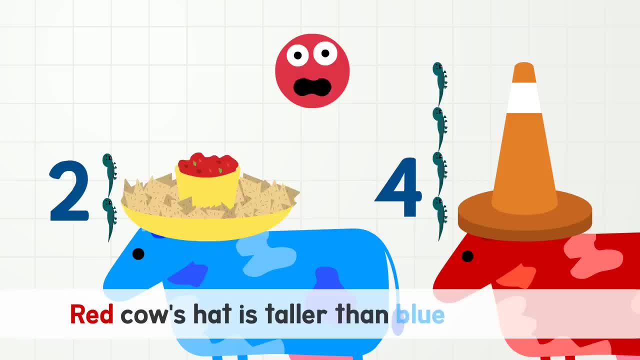 Four is a larger number than two. So that means that red cow's hat is taller than blue cow's hat, And the opposite is also true: blue cow's hat is shorter than red cow's hat. Now, if we look at yellow cow's hat, it is five. 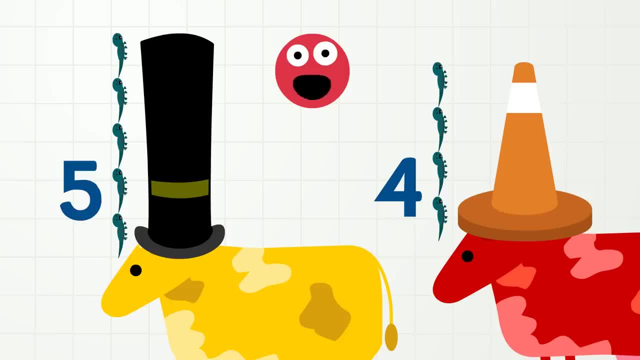 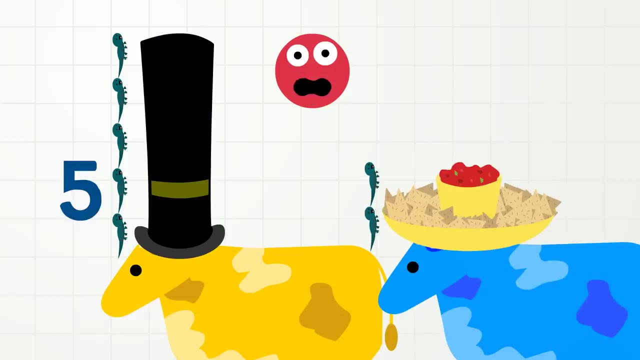 salamanders high Five is a larger number than four, so this means that yellow cow's hat is taller than red cow's hat, and the opposite is also true: Red cow's hat is shorter than yellow cow's hat. and five is also a larger number than two, which means that, out of all of the cow's hats that you 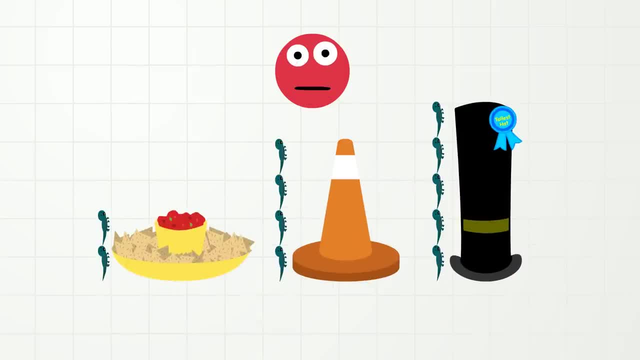 can see. right now, yellow cow's hat is the tallest hat- Taller hat, Tallest hat. Yay, Okay, good job. Now that you're getting better, let's measure how wide each of the cow's hats are. We call this the. 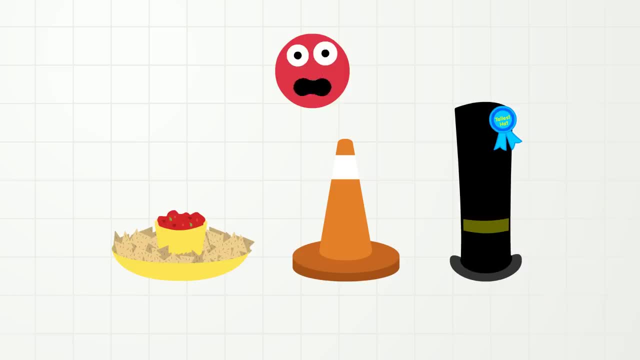 width, Width. And instead of measuring up, we will measure the width of each of the cow's hats. We will measure from side to side, From left to right. Ready, Let's go. So how many salamanders wide is blue cow's hat? 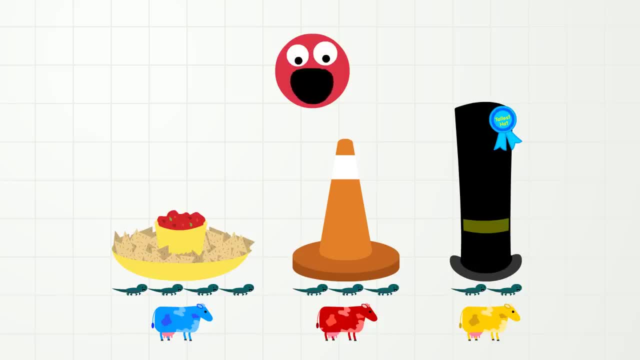 And how many salamanders wide is red cow's hat And finally, how many salamanders wide is yellow cow's hat. So which cow has the widest hat? Okay, that is all the time today we have for measuring, And remember that you can measure things too, like right after this video is over. 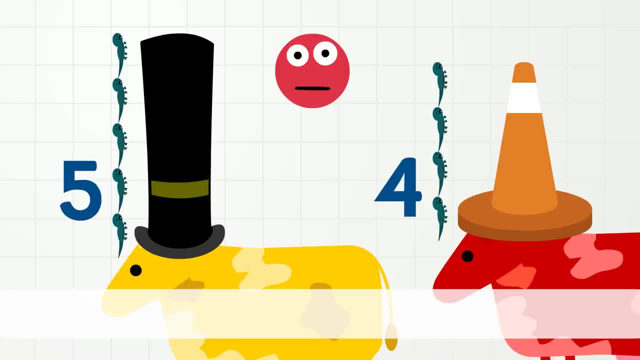 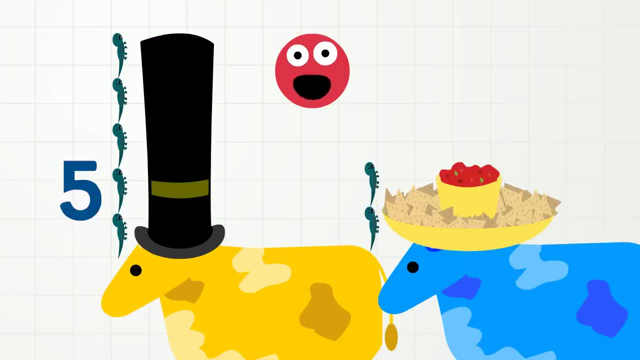 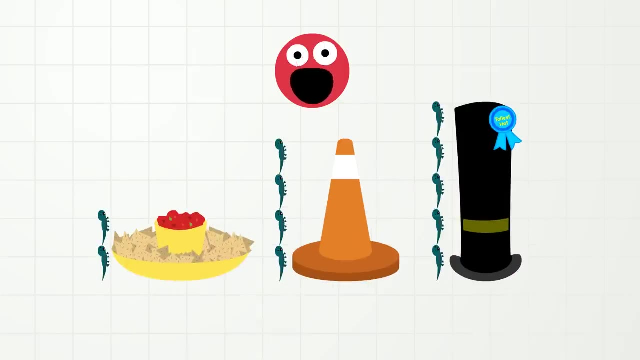 red cow's hat, And the opposite is also true. Red cow's hat is shorter than yellow cow's hat, And five is also a larger number than two, Which means that yellow cow's hat is taller than red cow's hat. Out of all of the cow's hats that you can see right now, yellow cow's hat is the. 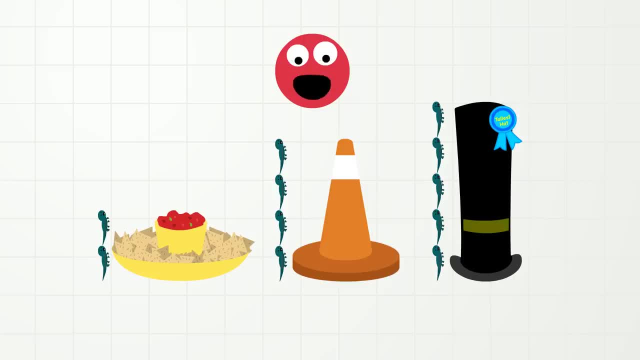 tallest hat. Taller hat- Tallest hat. Yay, Okay, good job, Now that you're getting better, let's measure how wide each of the cow's hats are. We call this the width Width, And instead of measuring up, we will measure from side to side, from left to right. 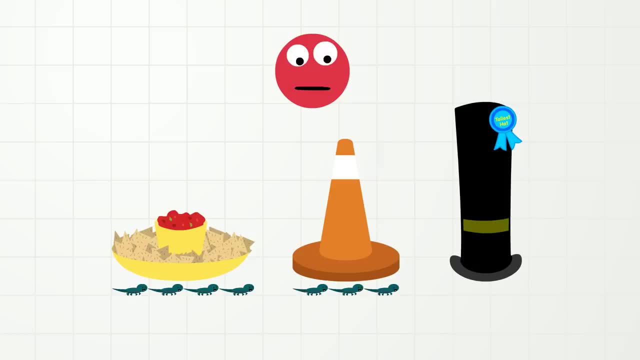 Ready, Let's go. So how many salamanders wide is blue cow's hat? And how many salamanders wide is red cow's hat? And finally, how many salamanders wide is yellow cow's hat? So how many salamanders wide is yellow cow's hat? 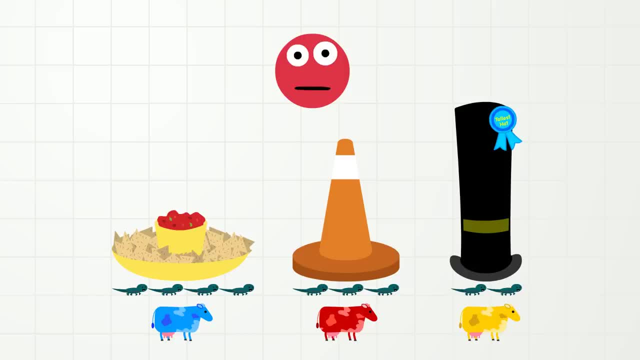 And finally, how many salamanders wide is red cow's hat, And finally, how many salamanders wide is yellow cow's hat, And finally, how many salamanders wide is yellow cow's hat. So which cow has the widest hat? 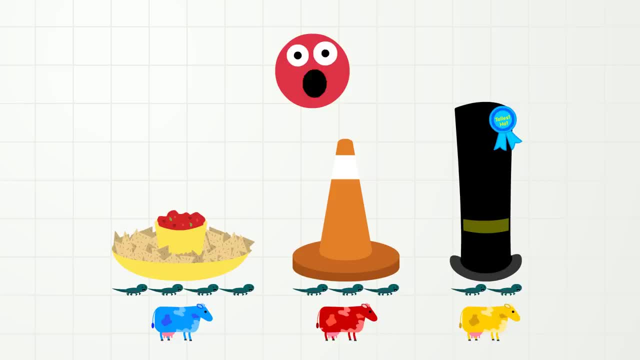 Okay, that is all the time today we have for measuring, And remember that you can measure things too, like right after this video is over, and even if you don't know any cows with funny hats And if you don't have any salamanders to measure with, you can use other things like rulers. 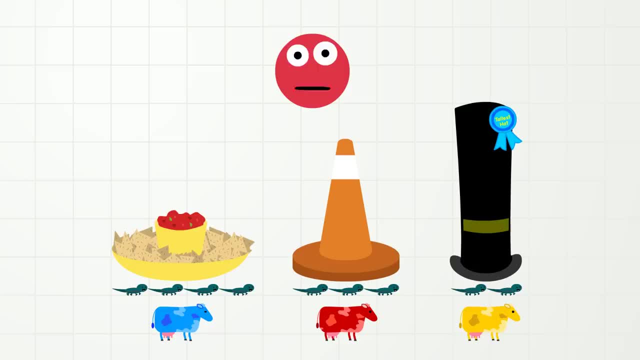 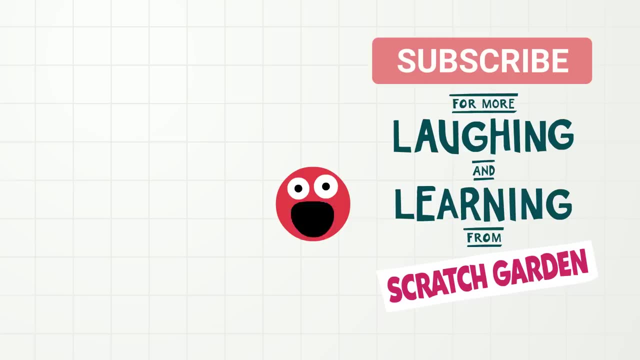 or erasers, Or even your feet. I wish I had feet. Anyway, don't forget to subscribe to our channel for more laughing and learning from Scratch Garden. Did you know that we have many, many videos with salamanders? No, it's true. Our salamander videos have created an. 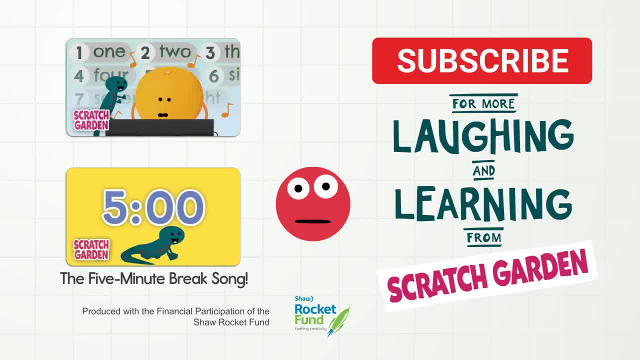 immeasurable amount of happiness for many, many people. Okay, bye for now. 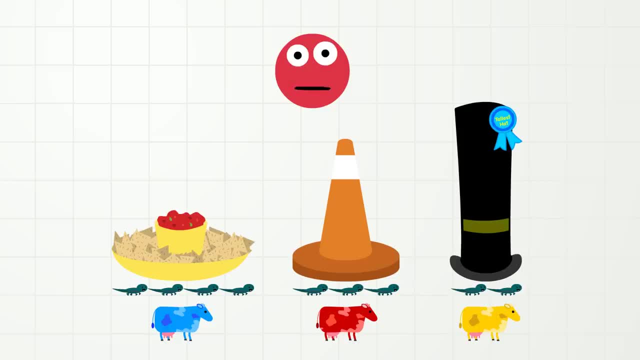 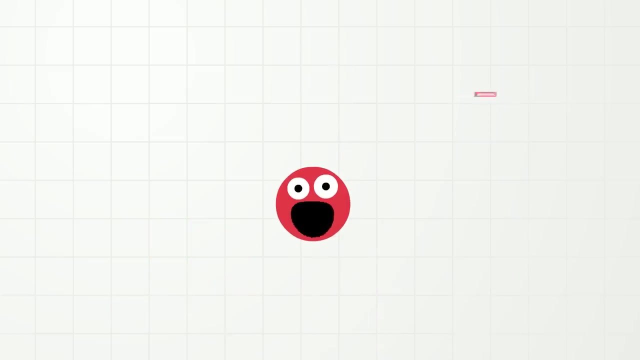 and even if you don't know any cows with funny hats, And if you don't have any salamanders to measure with, you can use other things like rulers or erasers, or even your feet- I wish I had feet. Anyway, don't forget to subscribe to our channel for more laughing. 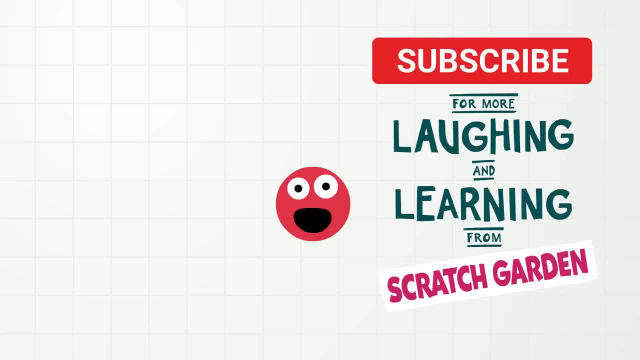 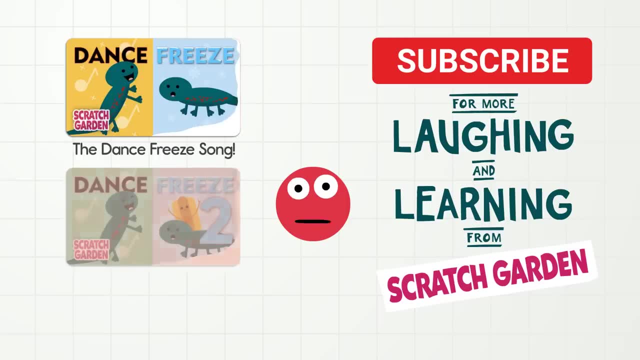 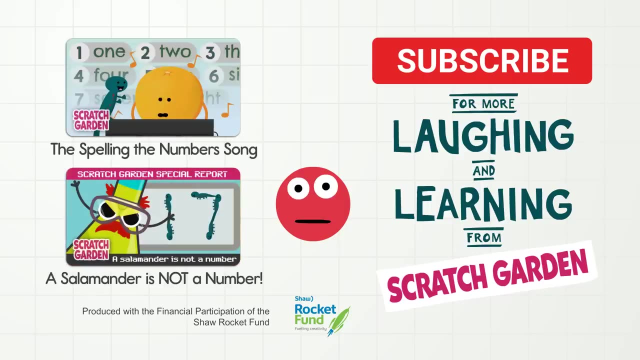 and learning from Scratch Garden. Did you know that we have many, many videos with salamanders? No, it's true. our salamander videos have created an immeasurable amount of happiness for many, many people. Okay, bye for now. Subtitles by the Amaraorg community. 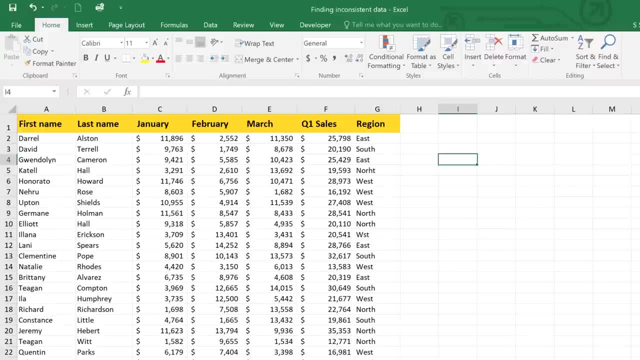 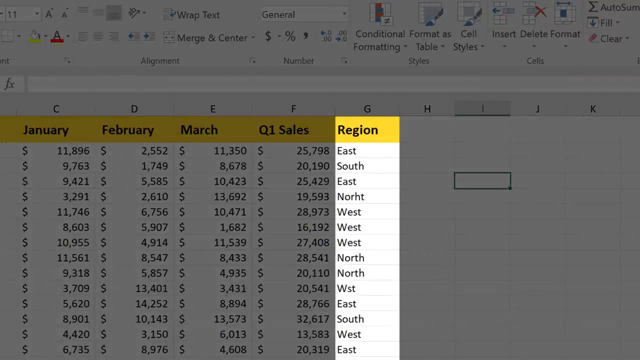 In Excel, details matter. If you have minor inconsistencies in your data, it can actually cause major problems later on. For example, I have a list of salespeople and each one falls into one of four regions: North, south, east or west. But if you look closely you can see that 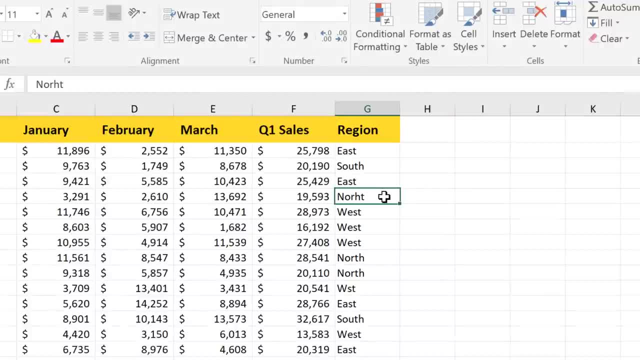 a couple of the values are a little bit different. It looks like north is misspelled and west is also missing an e And, believe it or not, these small differences might actually cause us to get the wrong result with certain formulas or pivot tables. Now, since we have about 300 salespeople, 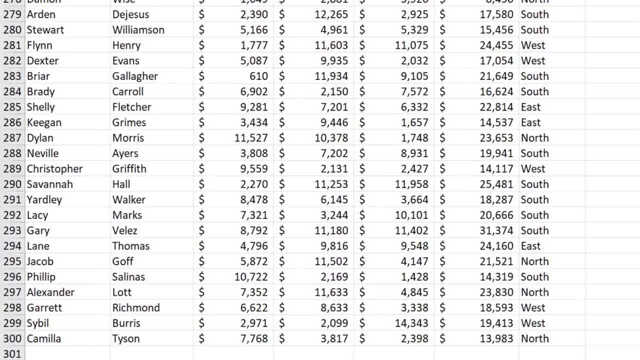 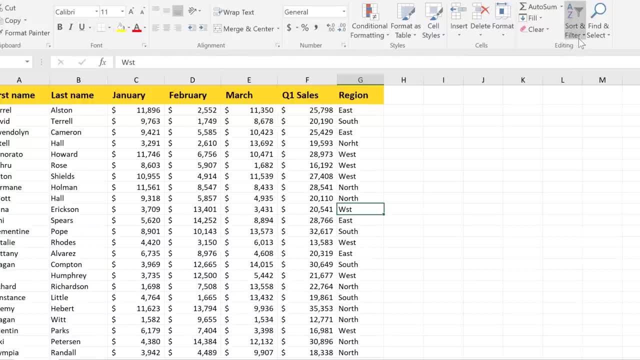 finding all of the inconsistencies would be like finding a needle in a haystack, But I'm going to show you a shortcut that's going to make it a lot easier. First, we'll need to apply a filter to the data, and you can get there from the sort and filter.